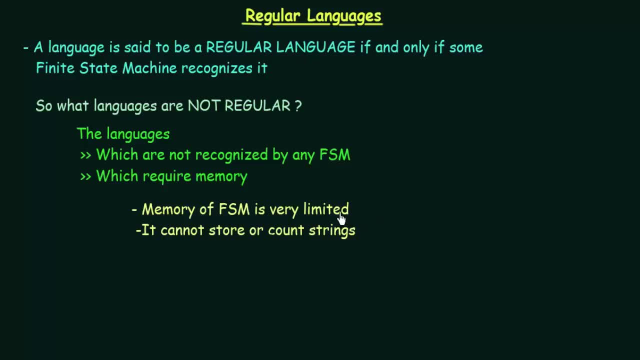 That is the only kind of memory it has. It doesn't have any other kind of memory. So its memory is very limited and also it cannot store or count strings. So the languages that requires memory or the languages that requires storing or counting of strings, 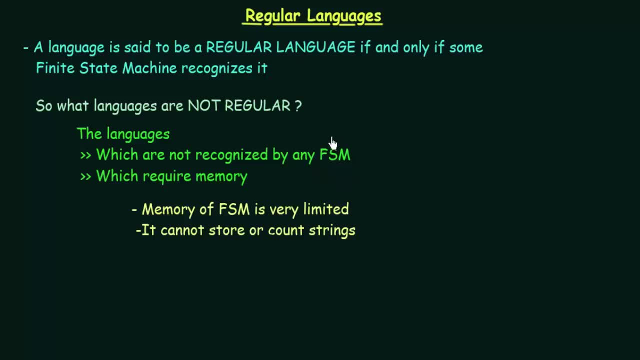 cannot be designed or recognized using a finite state machine, making it a language that is not regular. Alright, So I hope that was clear. So let us take a few examples to make it more clear. For example, suppose I have a language of this form: ABABB, followed by ABABB. 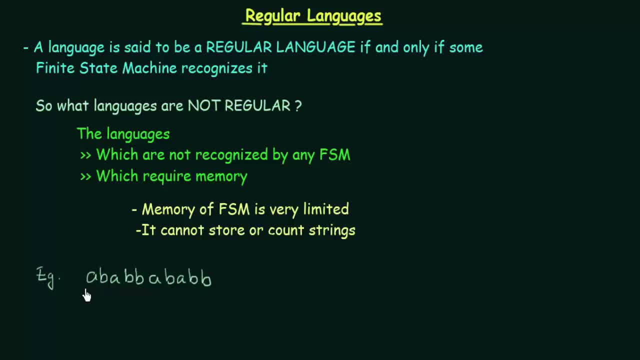 So what is the rule that this language follows? The rule that this language follows is that the first five letters, ABABB, is repeated again ABABB. So these five letters should be repeated. Exactly the same thing should be repeated again. That is the kind of rule this language follows. 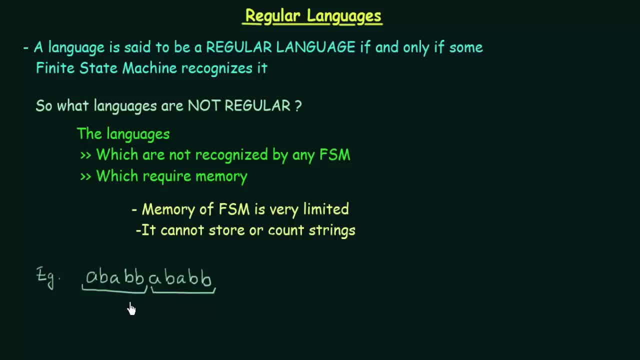 So let us see if this can be designed using a finite state machine or not. We see that, in order to repeat what was here over here, we need a memory which stores the information about this string Right. Only if we know what is stored here, only if we have the information about this. 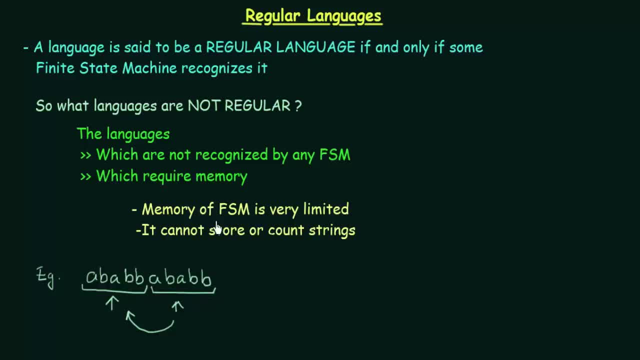 then only we can repeat it over here. But we know that finite state machine has a very limited memory, So it cannot store this part in memory so as to repeat it again over here. So this cannot be designed using a finite state machine, making it a language that is not regular. 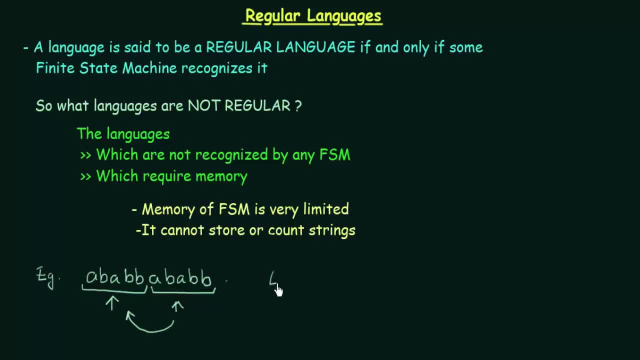 Okay, Now let me take another example. In this example, I have another language of this form: A power N, B power N. Now, what is the meaning of this? This means that the number of A's should be equal to the number of B's. 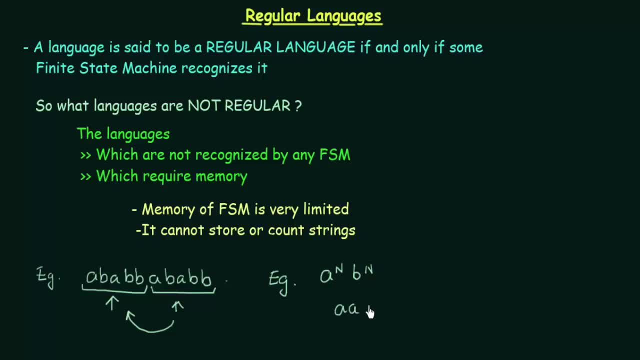 So suppose I have A, A, A, Three A's, Then it should be followed by B, B, B, Three B's, Because N should be same. That means the number of A's and number of B's should be exactly same.